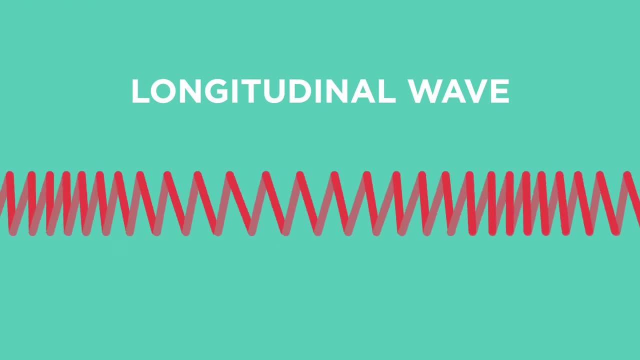 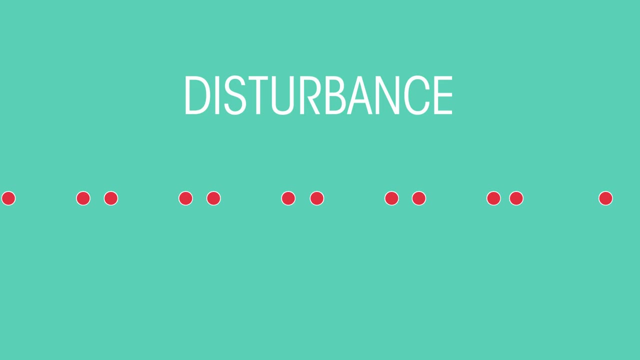 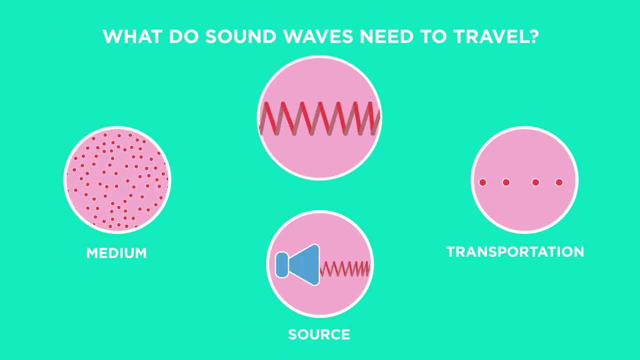 longitudinal wave pulsing like a slinky. Sound waves are technically a disturbance because they travel by disturbing the next particles along. What does sound waves need to travel? Sound needs a medium to travel through, because it needs particles to travel through. Sound waves are: 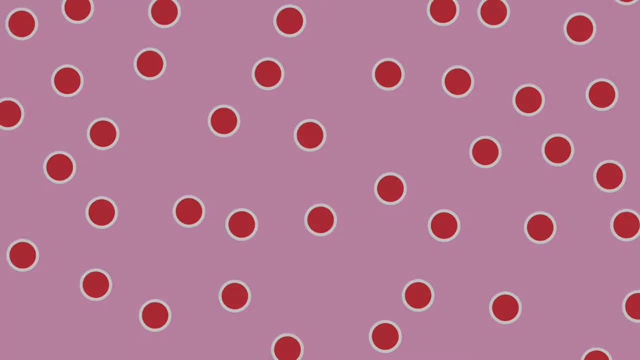 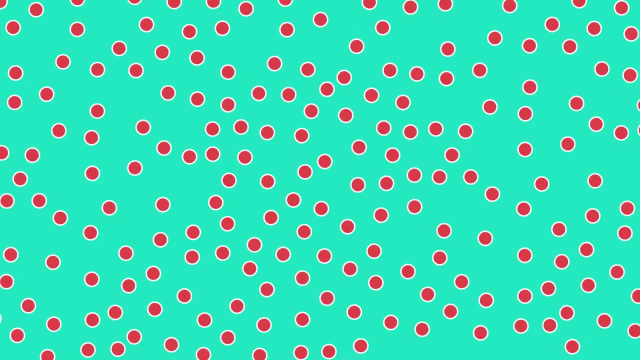 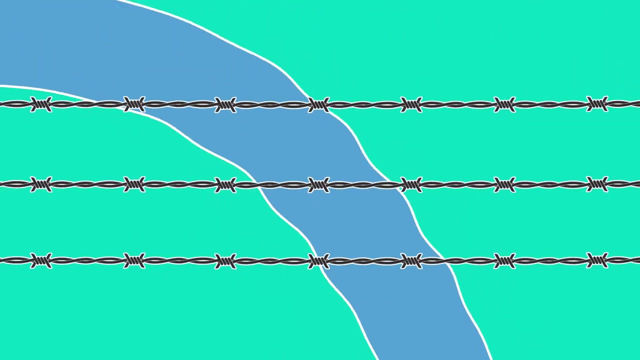 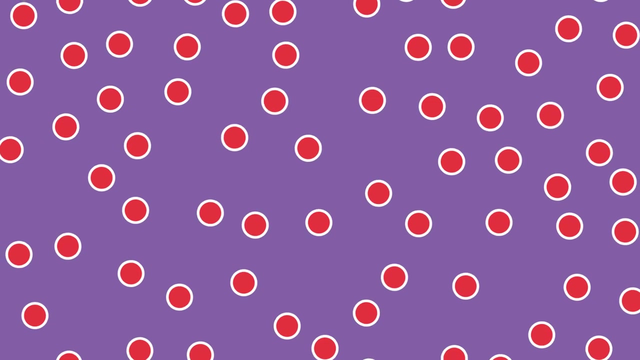 to disturb, which is why the vacuum of space is silent. There are no particles for sound waves to disturb. Usually this medium is air, though it could be any material such as water or steel or the ground. The medium is any series of interconnected and interacting particles, So it can be solid. 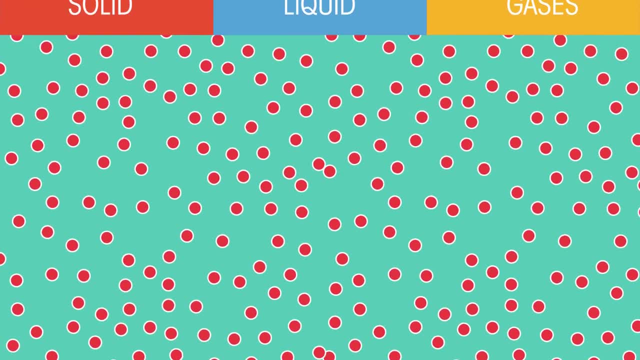 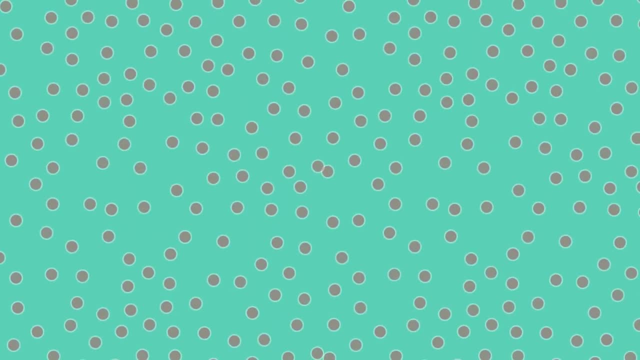 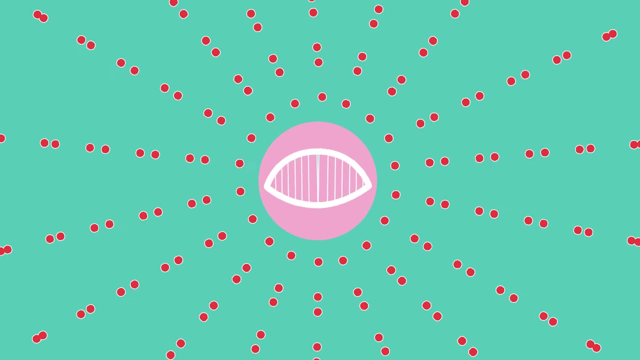 liquid or gas. So we have a medium. Sound then needs an original source of the wave. The source is any vibrating object that can disturb the first particle of the medium. The disturbance could be vibrating vocal cords, the vibrating diaphragm of a speaker or the vibrating metal of a machine. We have our 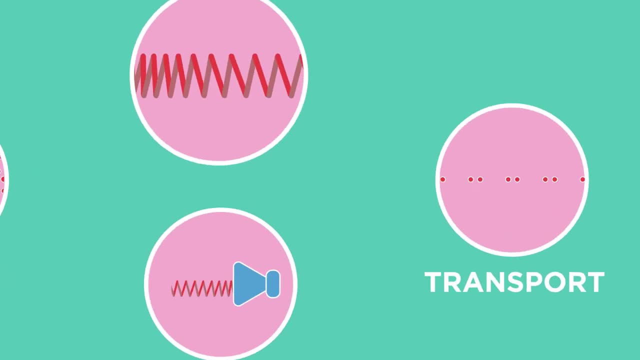 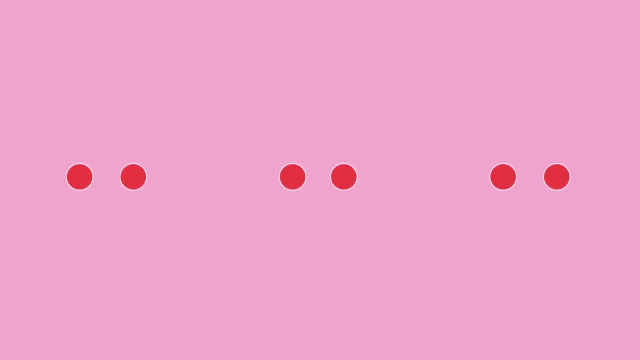 source and our medium to travel through. The sound wave is transported from one location to another by practical to particle interaction. As one particle is displaced, it exerts a push or a pull on its nearest neighbours, causing them to be displaced from their position. The Rubins tube is a spectacular physics experiment involving fire to demonstrate that sound is a. 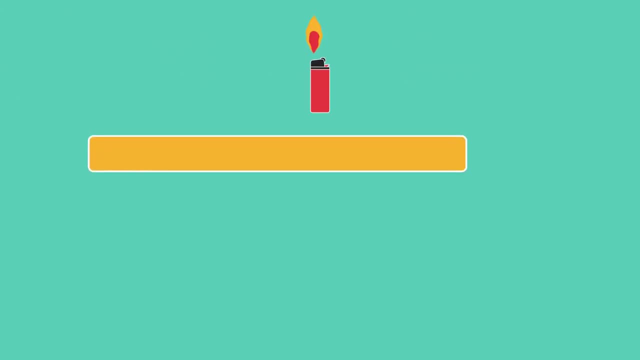 longitudinal wave tube is a hollow tube that is filled with a flammable gas, usually propane. holes are drilled at regular intervals along the top of the tube. one end of the tube has a rubber membrane stretched across it and a loudspeaker positioned next to it. the gas leaks through the holes at the top of the 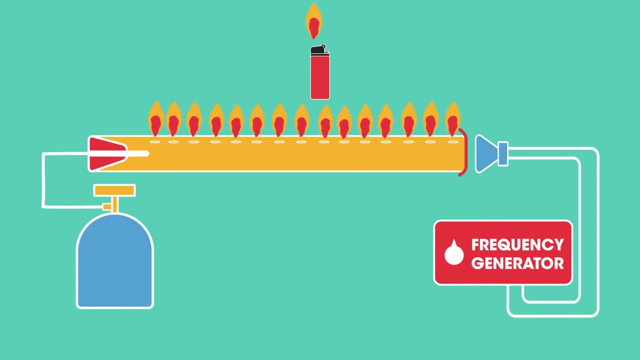 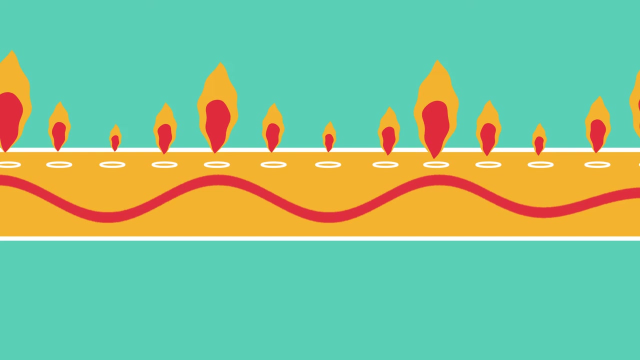 tube. the gas is lit, creating lots of small flames along the top of the tube. when the speaker is switched on, sound waves travel down the tube. the gas inside the tube follows the sound pressure wave and leaks out of the holes in a wave pattern. therefore, the flames also appear wave-like.